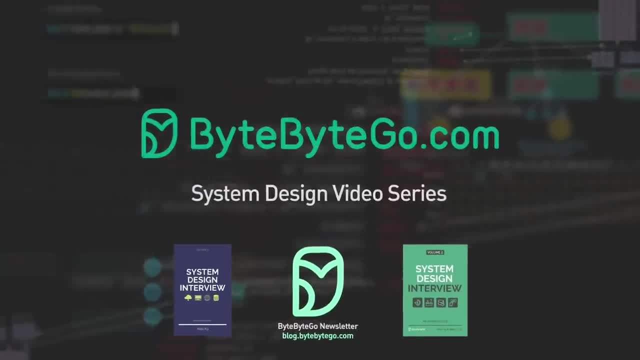 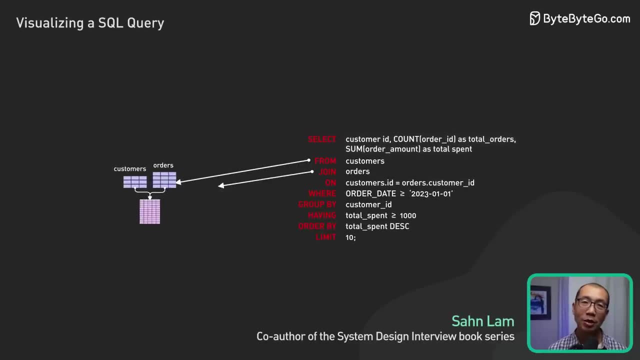 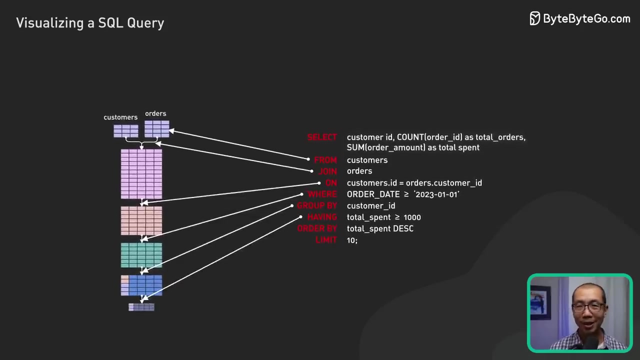 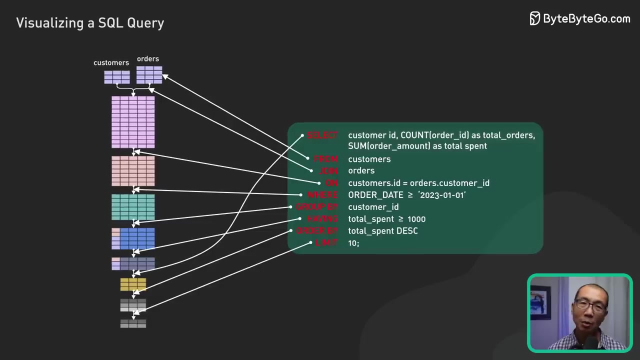 In this video we're going to deep dive into SQL query execution. We'll cover query processing optimization techniques and best practices. Let's get started. Here's the example query we'll use throughout this video. In this query we find the top 10 customers with at least a thousand dollars. 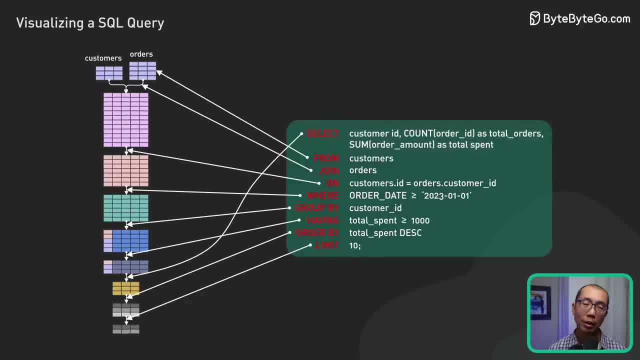 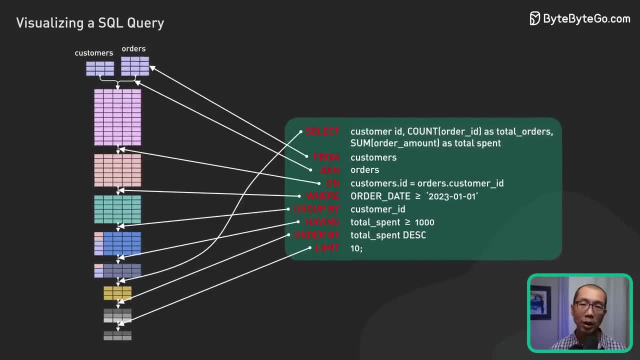 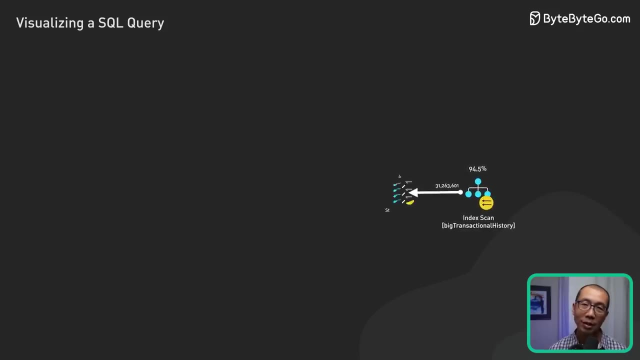 spent on orders since January 1st 2023. by joining the customers and orders table and grouping by customer ID, We display their total orders and amount spent, sorted in descending order by the total spent. Now, before we dive into the query, let's discuss query execution plans Database. 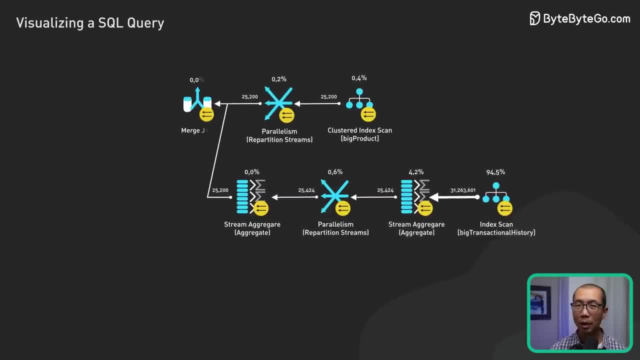 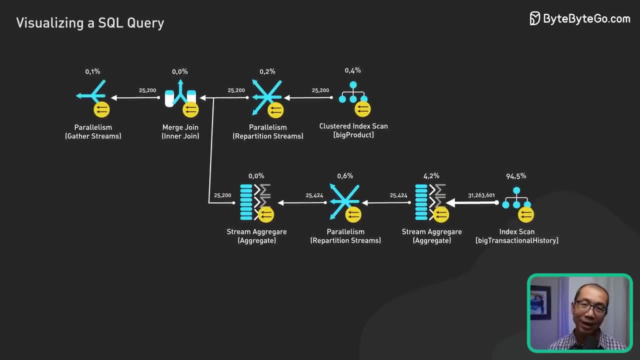 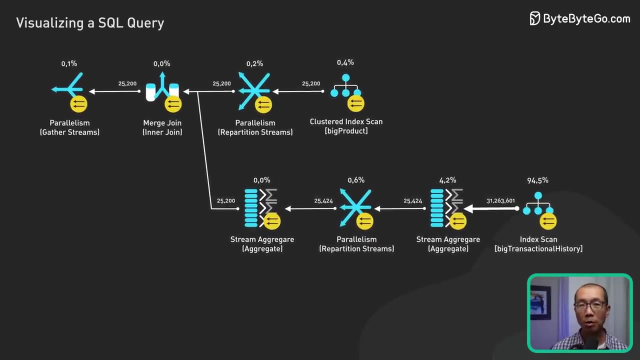 systems, create these plans to optimize queries and minimize resource usage. Understanding the plan can help us optimize our query for better performance. Execution plans provide information like estimated costs, chosen joined algorithms and a sequence of operations. Now, first let's start with the from and join clauses. This is where we choose the tables. 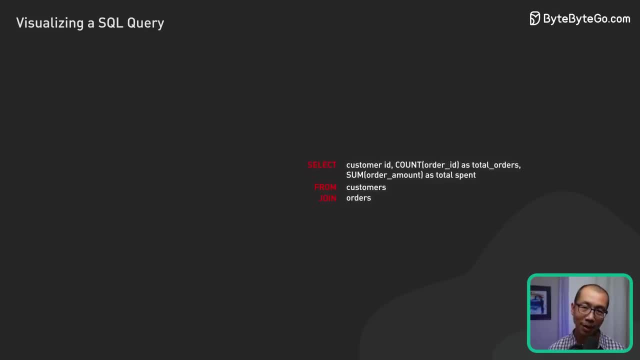 we want to work with and specify how to join them In our query. we are using the customers table and joining it with the orders table using the common ID and customer ID columns. Now, using indexes on join columns, we can see that the order table is the order table. Now we can see that the 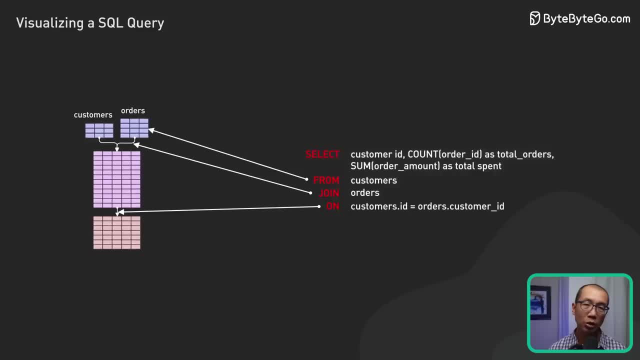 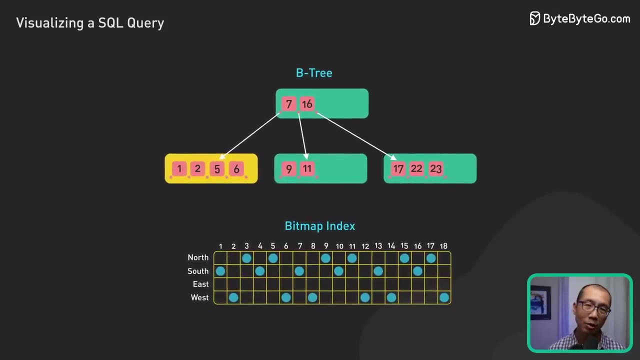 use of index and parse columns can significantly improve the performance of the join operation. Make sure we have appropriate indexes in place for faster query execution. Index types such as B3 and Bitmap indexes can impact performance based on data distribution and query types. Now we move to the WHERE clause. This filters the combined data. 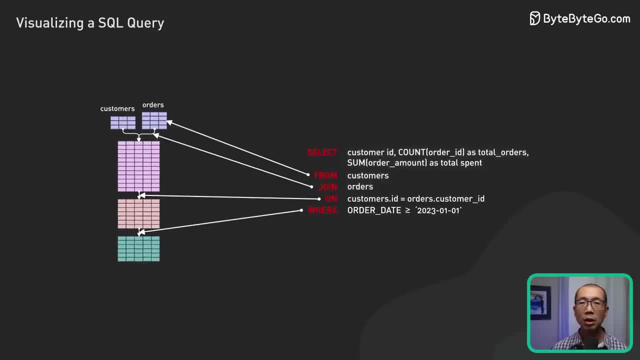 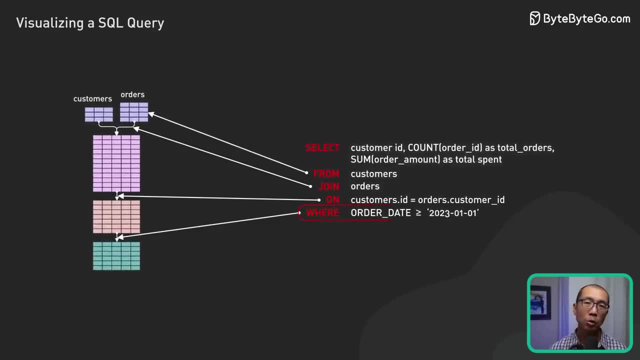 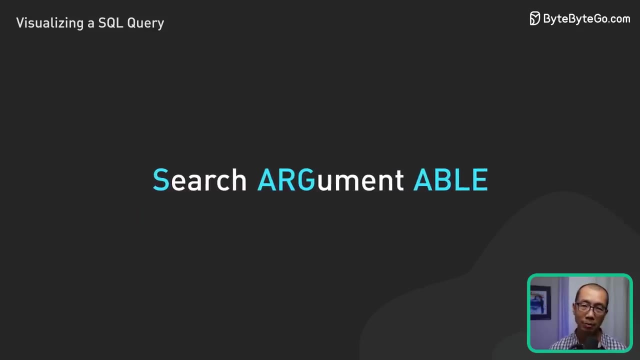 by applying a condition. In our case, we are considering orders placed on or after January 1st 2023.. Now it's important to write a solvable query to leverage indexes effectively. A solvable means search argument able And it refers. 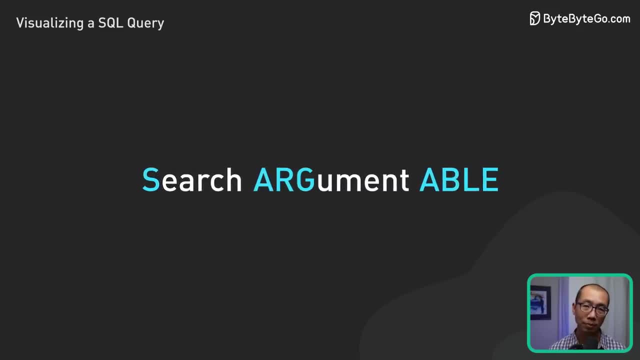 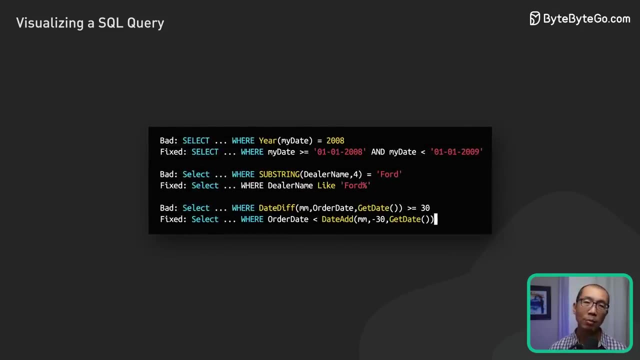 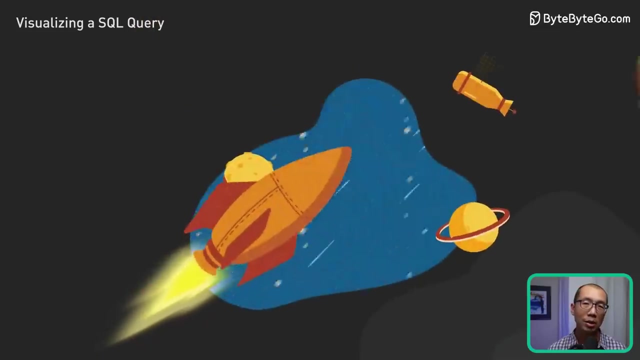 to queries that can use indexes for faster execution. Now let's dive deeper into the concept of solvable queries. When we say a query is solvable, it means that the query can efficiently use indexes to speed up the execution process. Writing solvable queries is essential for optimizing. 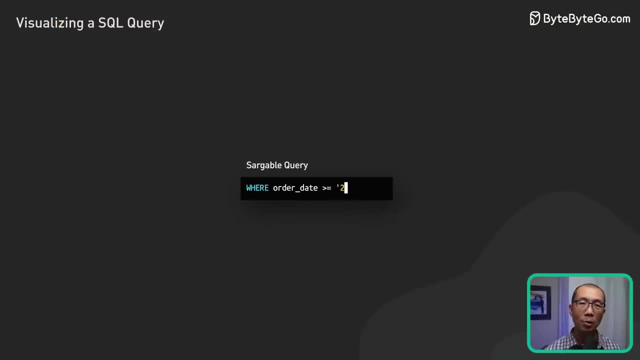 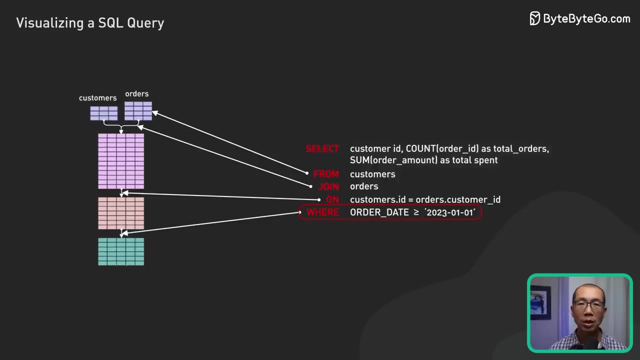 database performance. Now here's an example to help illustrate solvable versus non-solvable queries. In a solvable query, we directly compare the order day column to a specific date. This allows the database engine to use an index on the order day column to quickly filter out. 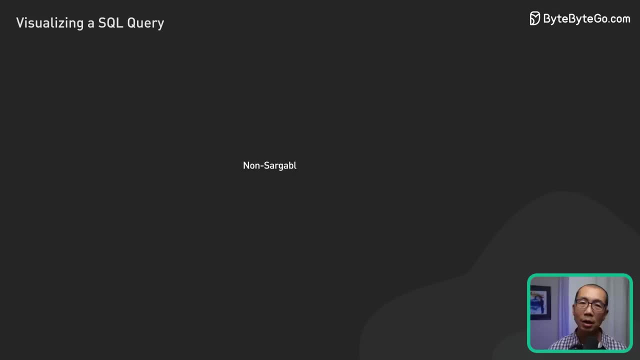 the records that meet the condition. In contrast, the non-solvable query uses the year function on the order day column. This prevents the database engine from using an index on order date because the function must be applied to every row in the table, even if 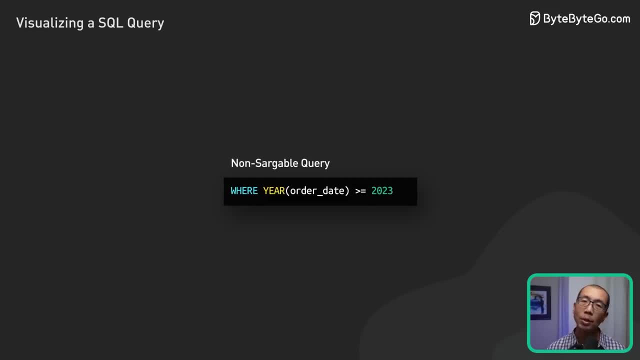 the index exists. The non-solvable query will be slower because there are a lot more records to scan. To write solvable queries: 1. Avoid using functions or calculations on index columns in the where clause. 2. Use direct comparison. 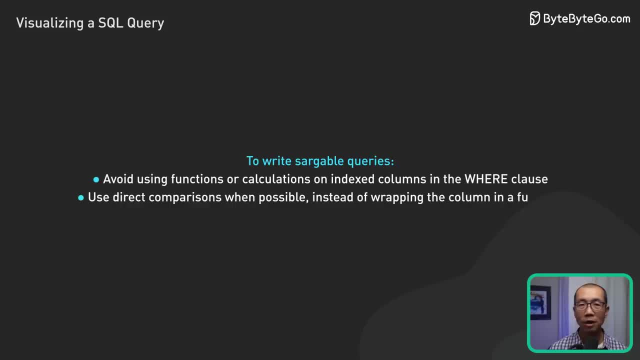 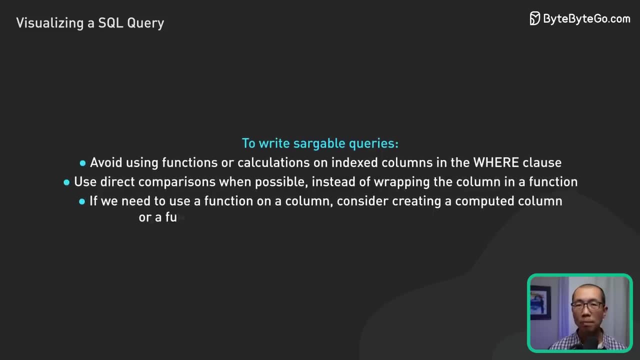 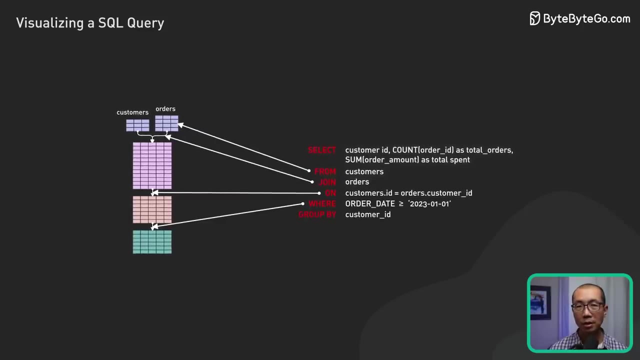 When possible, do not wrap columns in a function 3. If we need to use a function on a column, create a computed column or a function based index if the database system supports it. Next up are the group by and having clauses In our query, we are grouping the records by customer. 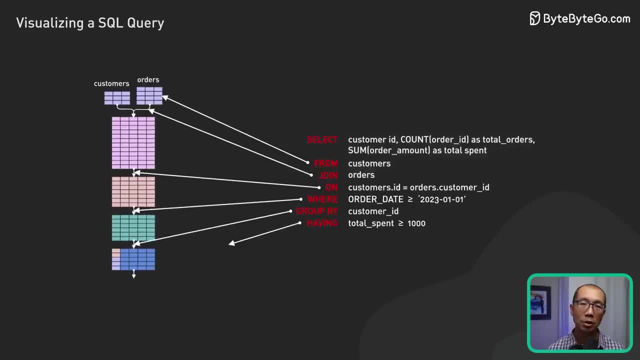 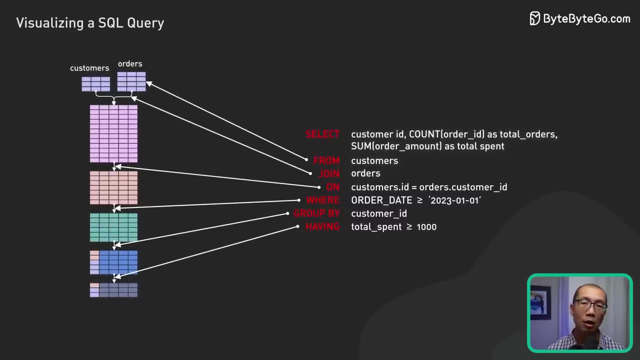 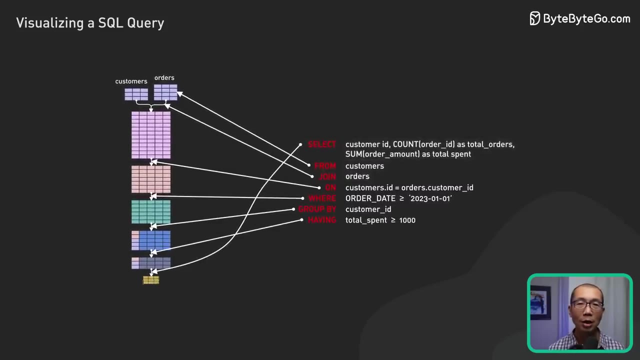 ID and filtering the groups based on the condition: total span greater than or equal to 1000.. This query finds those who have spent a significant amount on orders. The SELECT clause comes next. It defines which columns we want in our result set. In this case, we are selecting customer ID. 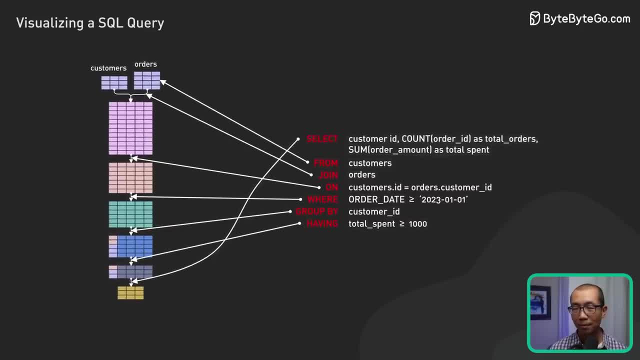 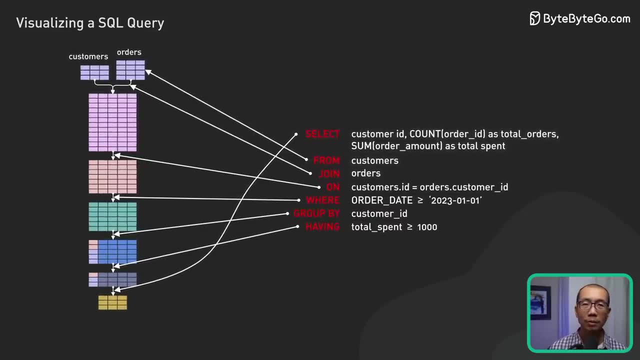 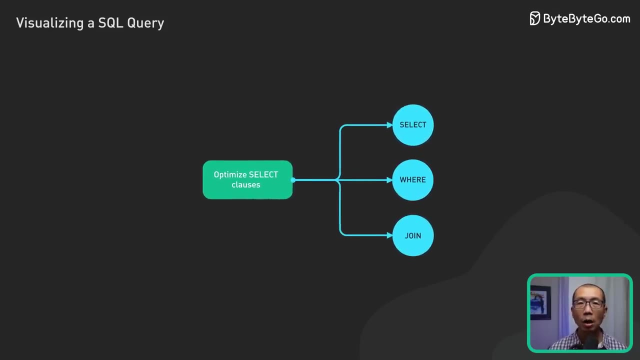 total orders and total spent. Even though SELECT comes first in a SQL query, it is pretty far down in the query processing order. When optimizing SELECT clauses, consider using covering indexes that include all the columns. The SELECT clause is used to identify the columns needed for. 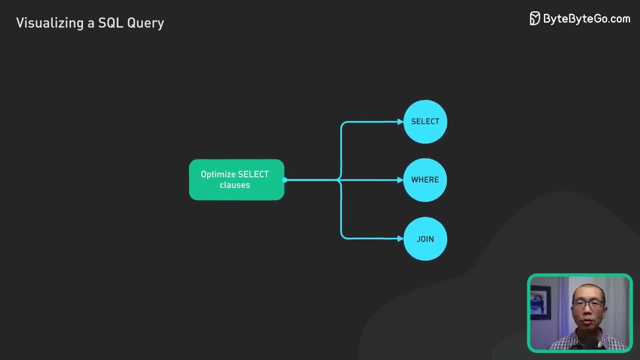 the query, especially in the SELECT, WHERE and JOIN clauses. This enables the database engine to retrieve data directly from the index. This speeds up query execution. Covering indexes can reduce the need for additional IO operations and minimize performance overhead.